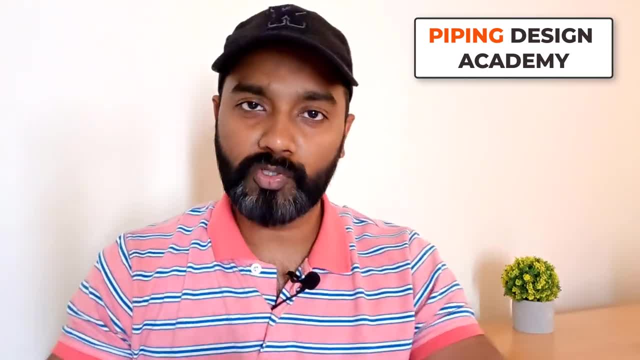 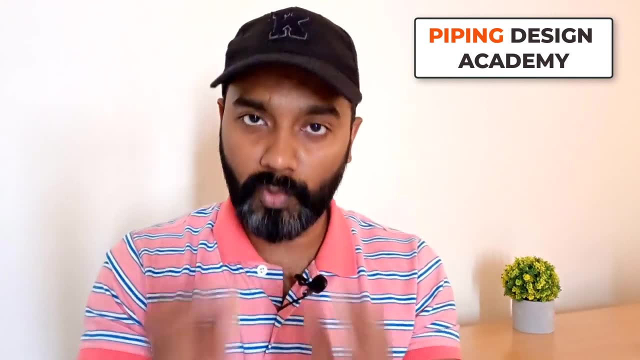 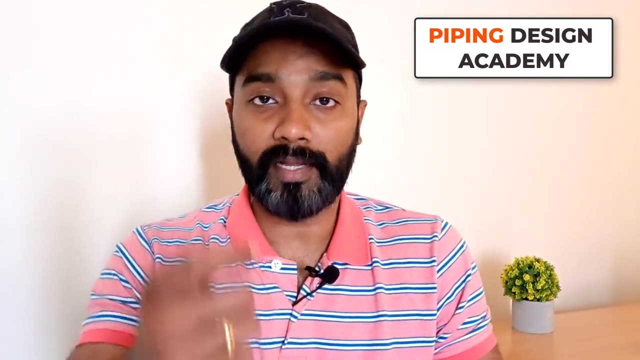 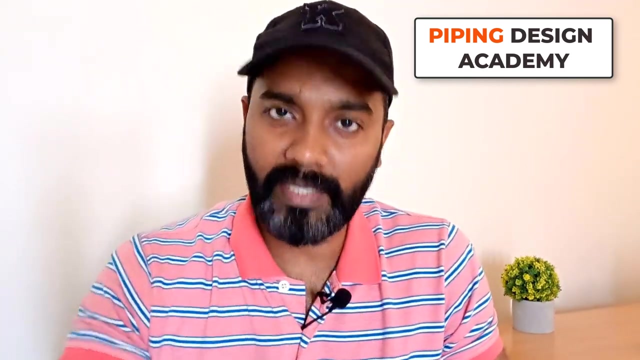 fail to understand the reality. That's when we used to spend a lot of time in unnecessary requirements. But once you understand the reality, you just have to focus on those reality requirements so that you will meet the requirement of industries. And the information that I'm going to share in this video is true to my knowledge, and nothing more or nothing less is expected from the industries, And if you meet these requirements, you can get into piping design engineering field. So with this, 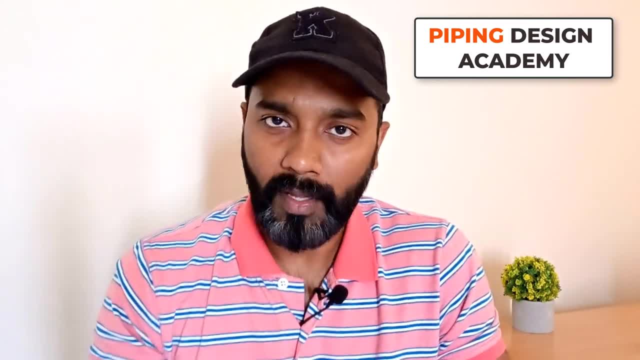 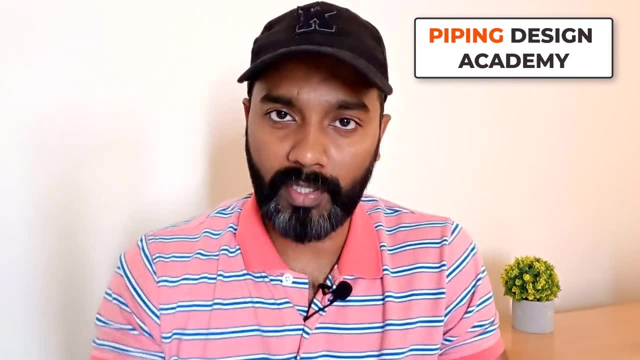 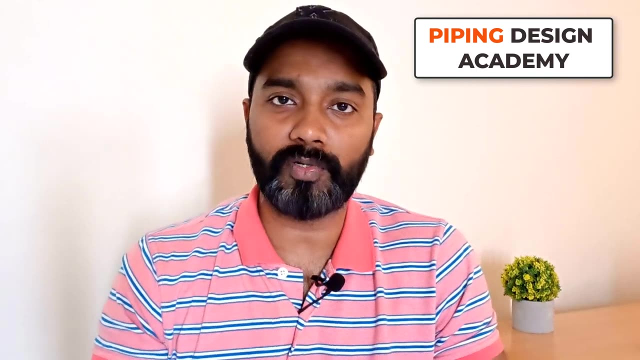 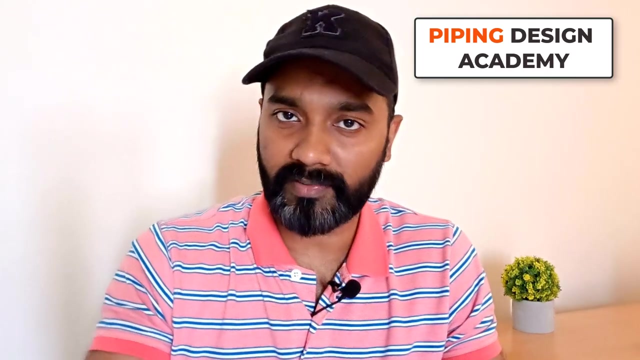 let's start from the first step that you have to do. So the first step for any beginners or anybody who are interested in piping design engineering should do is you should understand the purpose of design. Why do we design? What is the requirement for this industry? So this is a big process plants industries and the process plants are known for manufacturing chemicals and petrochemicals and various other byproducts. So the core 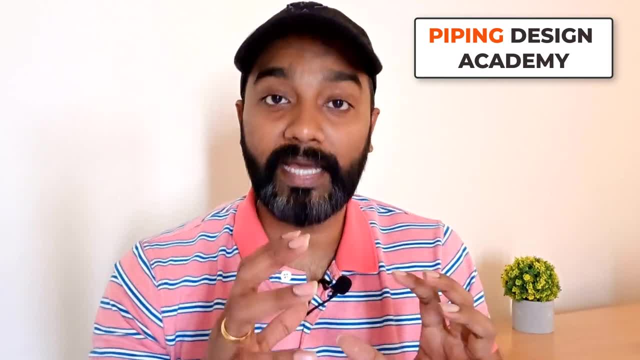 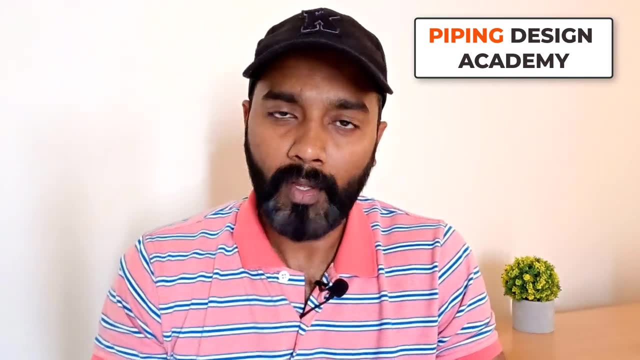 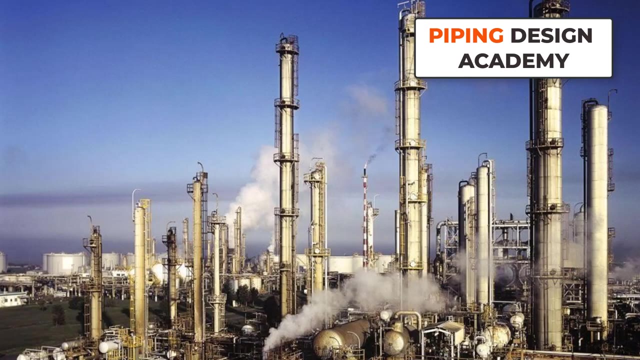 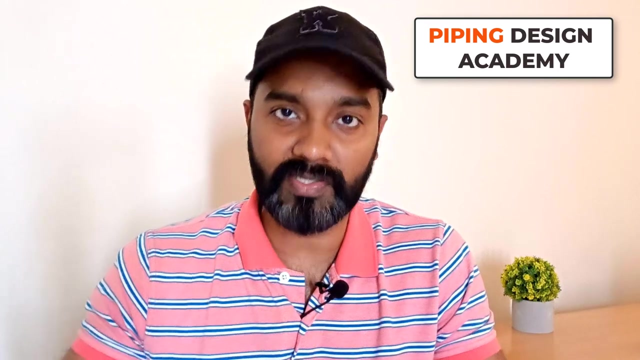 value of piping design is to facilitate and build the infrastructure for piping so that these manufacturing can be enhanced and facilitated. So your ideal purpose of doing a design is that you're trying to build something which is useful for the manufacturing industries, And these manufacturing industries are known as oil and gas, petrochemicals, fertilizers, power plants and these things. So piping is the core part of this process. 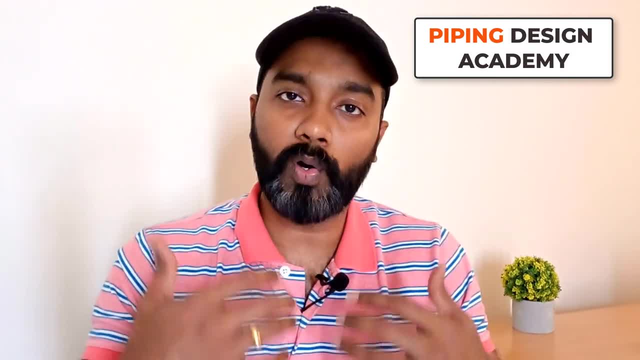 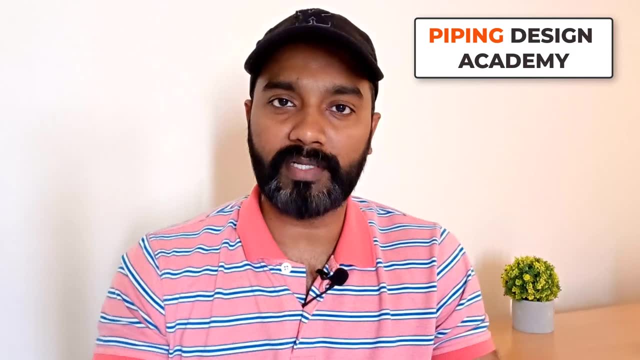 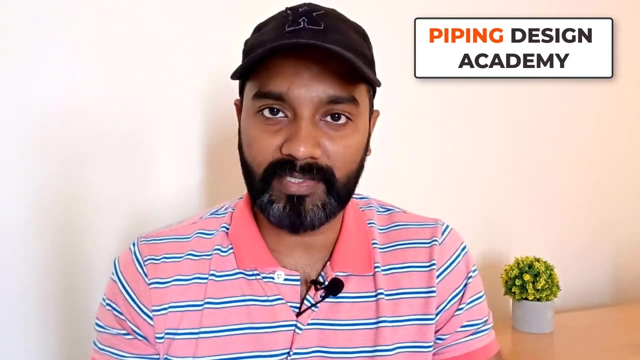 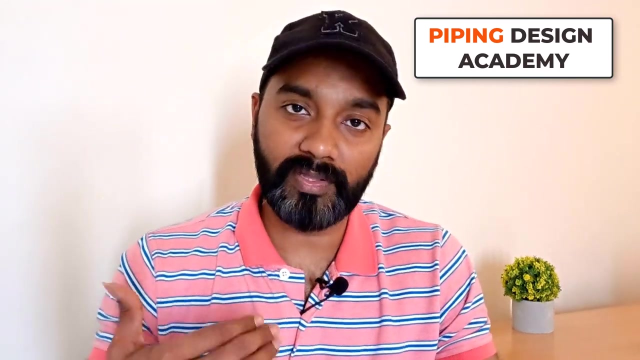 as long as you have this process plans, you don't have to worry about anything. you will have opportunities, you will have scope for design. So you, as a beginner, to need to understand what is the purpose of your design, what is the purpose of your like being a piping design engineering for this world. that you have to understand first, actually, because only then you will be able to relate yourself with this field. If you don't understand what you're doing and why you're doing, and it's completely useless, right? 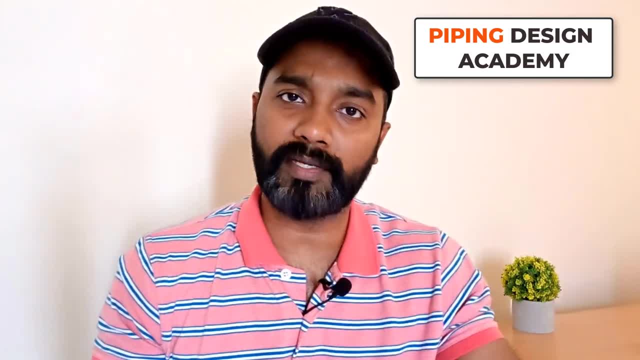 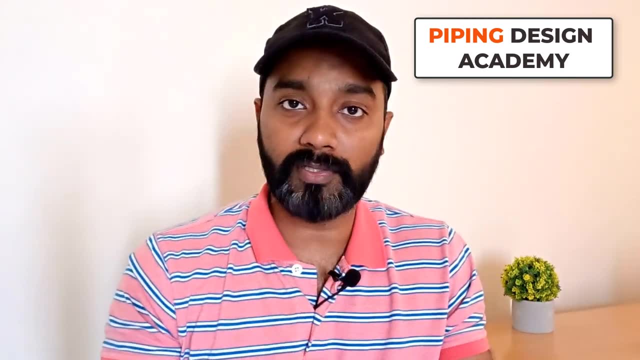 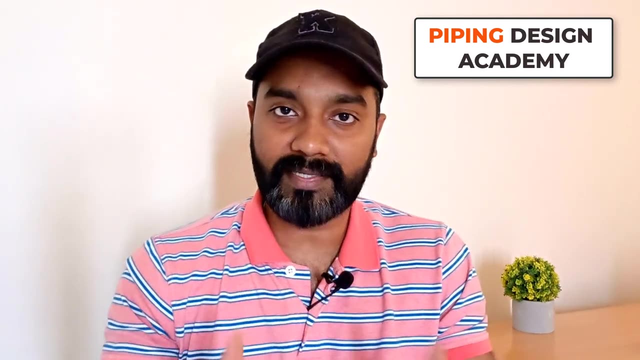 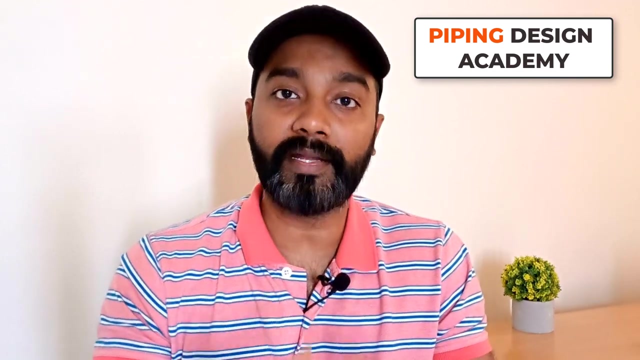 Say, for an example, being an automobile engineer, if you don't know anything about what you're going to deliver, and it's not the right way of thinking. right, Being an automobile engineer, you should know about this vehicles, what you're going to produce and what is your role basically. So for that you have to understand the intent of this particular role. So the intent of piping design engineering role is to facilitate and build the constructive infrastructures for any process plant requirements. 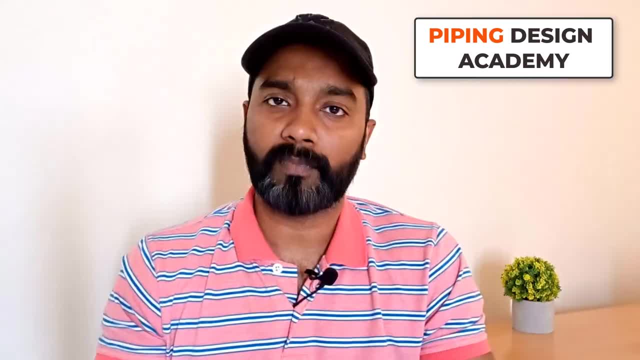 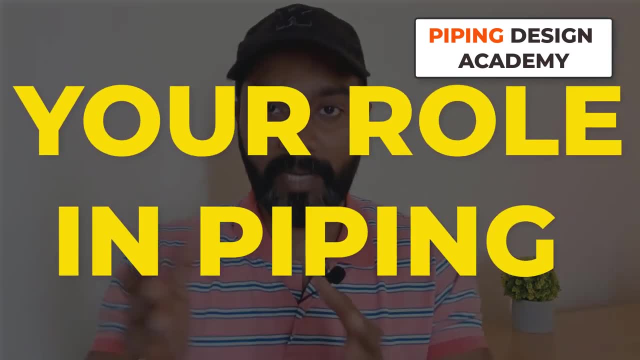 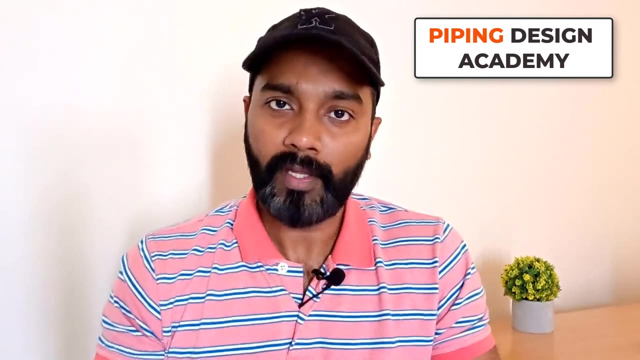 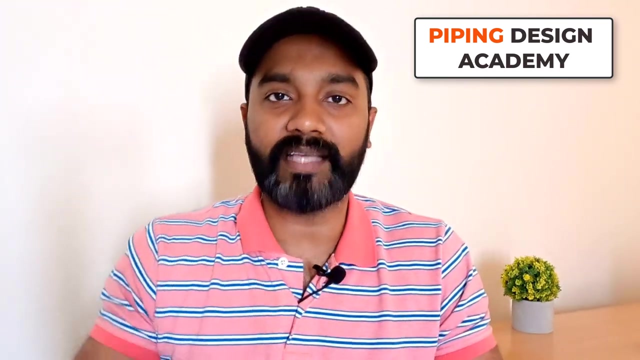 So now let's get into the step two. The step two is: we know the purpose of the design, but what is your role? You have to understand your role as a piping design engineer in this particular industries, What you're being expected to do it. actually, you know that you're going to deliver this piping design and those things, But what is your role? Your role is to manage the design. your role is to get the inputs and what you call deliver the output. 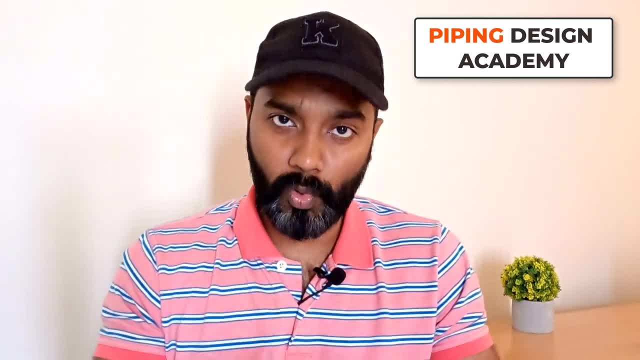 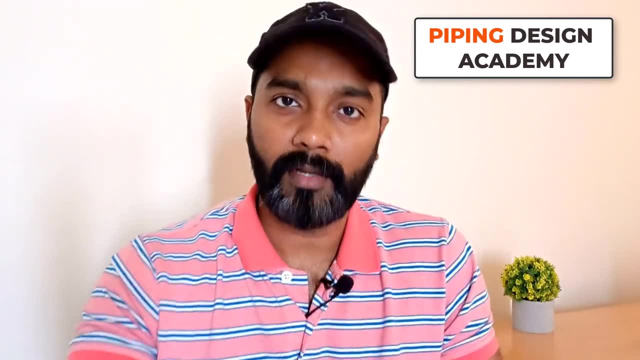 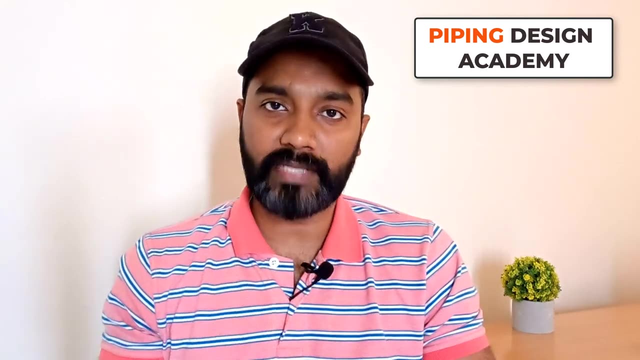 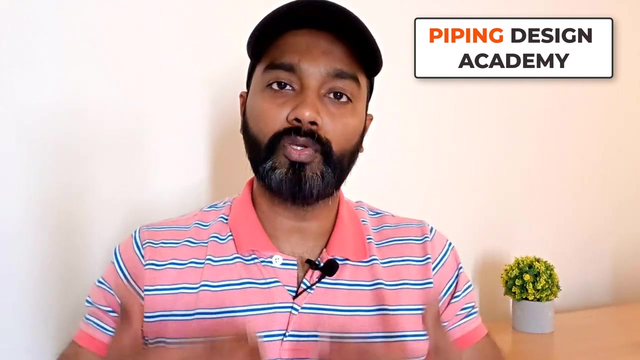 That are expected from clients. So your role is to design this entire thing from scratch. For that you have to follow the standards, you have to follow the some specifications, you have to prepare drawings, you have to prepare a 3d model. there are lots of coordinations, activities that you have to do. So for that you need to know what is your role is about actually. So if you do not know your role, you cannot manifest yourself about who you are basically. 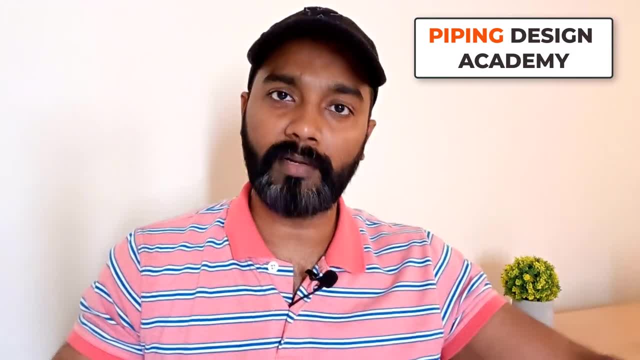 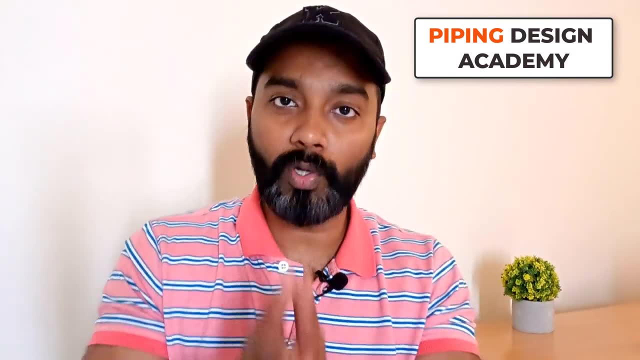 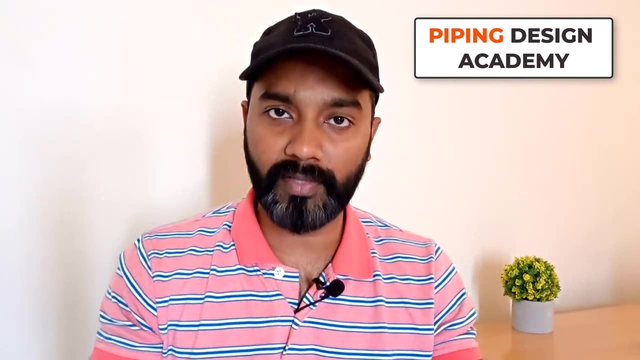 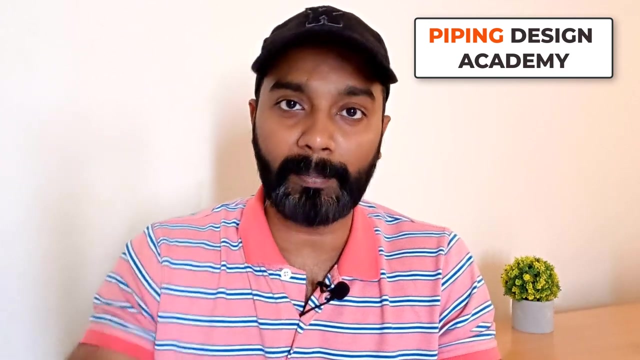 So you understood the industrial process. you understood the purpose of the industries and the purpose of piping design, but you also have to understand your role, Because your role defines who you are. So, as a second step, you guys have to understand your role. There are lots of materials available in the internet. Even if you search in my channels, there are lots of videos where I have explained what is the role of piping design engineers. That is more than sufficient for you to understand what, who you are and what you have to do. 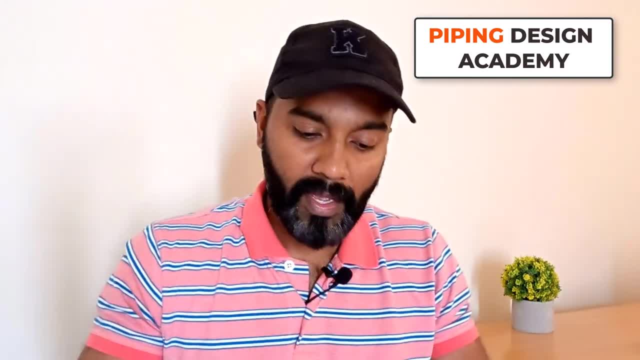 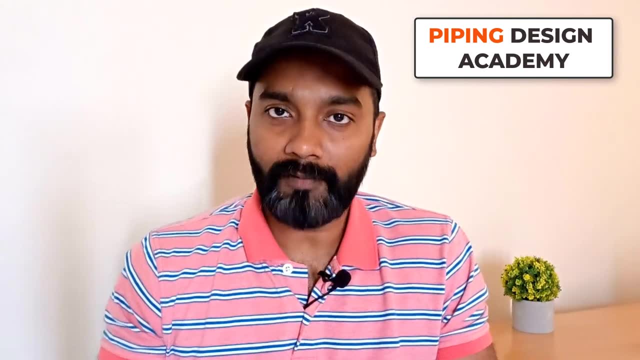 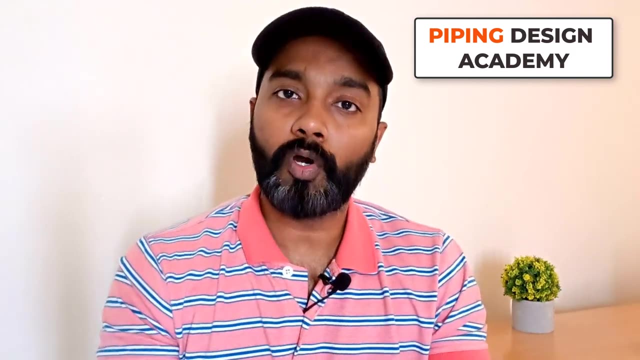 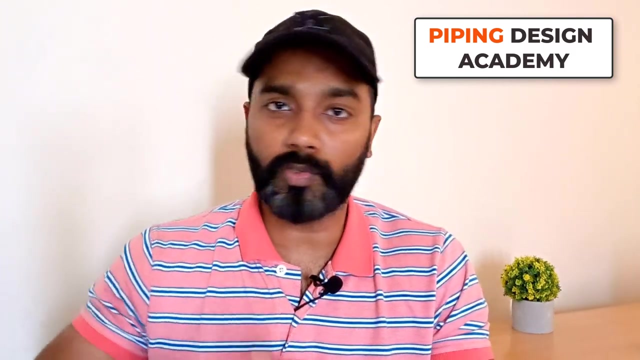 So this is the second most important thing, actually, And the third most important thing is that you have to understand the job criterias. See, you are preparing yourself as a piping design engineer, So you have to understand what is the job criteria. as a beginner, If you are looking at the criterias which are actually required for a 10 years and 15 years experience, you will be completely confused actually. 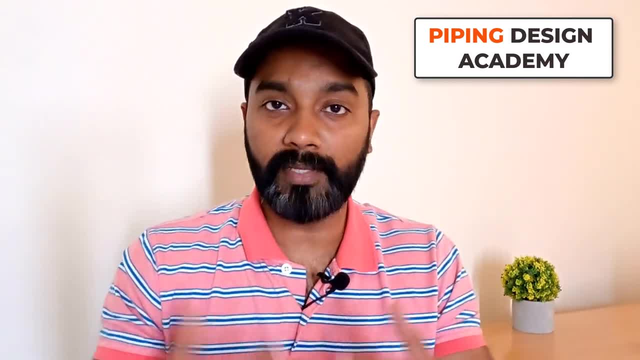 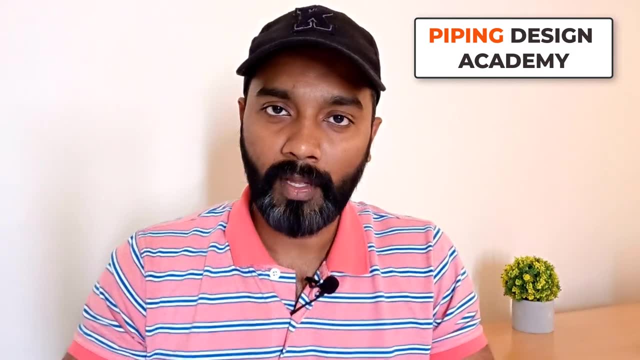 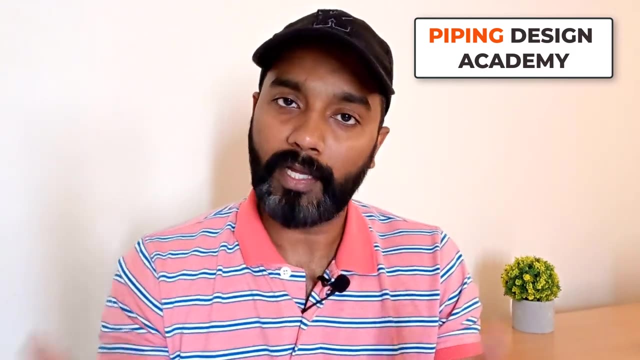 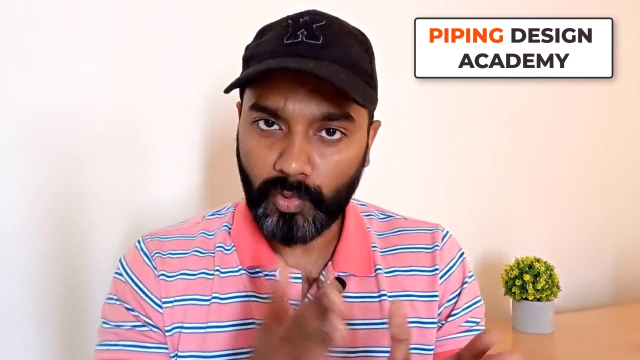 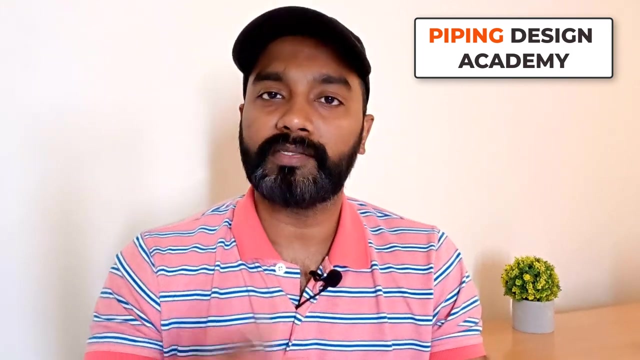 Being a piping designer and being a beginner- I mean being a beginner in piping- you have to understand what is the job criteria that are to be met for beginners. So this is very simple. If you just browse in naukricom, you will find a lot of opportunities. Look at the opportunities which is only called for beginners And then you will be able to understand the job criterias. So job criterias will be saying so that you will have to have a basic engineering qualification and some 2D softwares and piping design engineers. 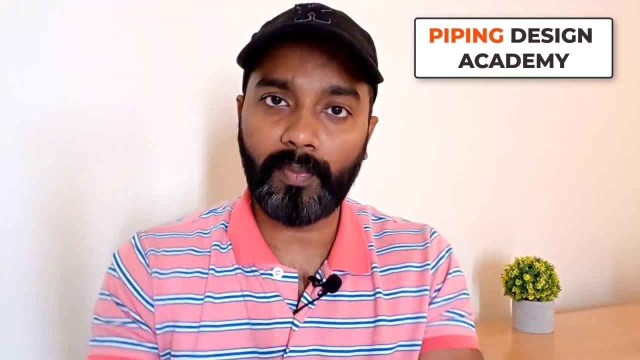 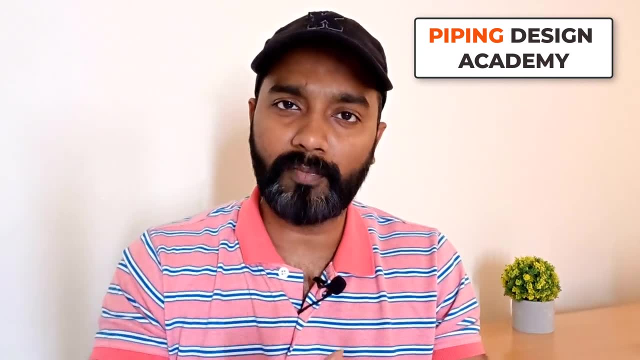 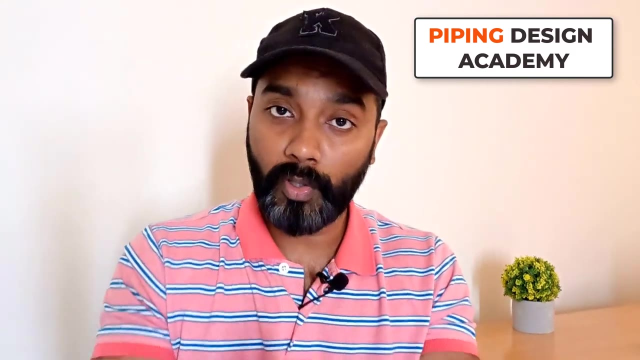 basics, those things you have to understand. in the next topic I will list down what you have to prepare actually. so if this job criterias, it varies companies to companies in a very minor fraction, but predominantly the job criterias are going to be same. so, as a third step, your duty is: 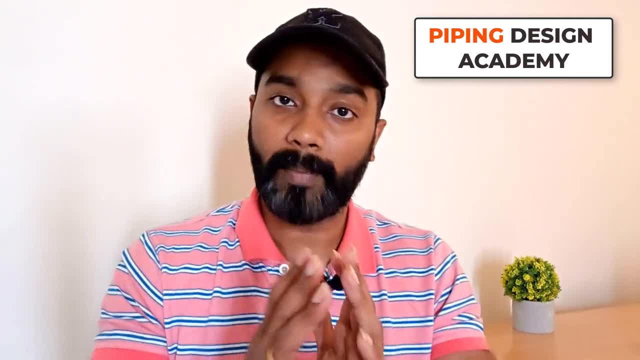 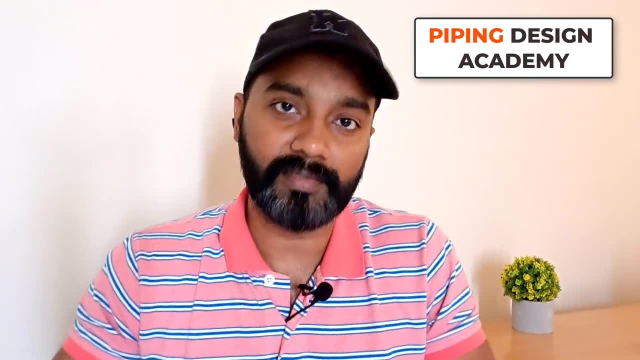 to check your job criterias. for that naukri can help you. by browsing in naukri, spending some time and going through multiple job positions, you will be able to understand your job criteria. so these are the things that you have to do. it actually simply just when somebody has suggested. 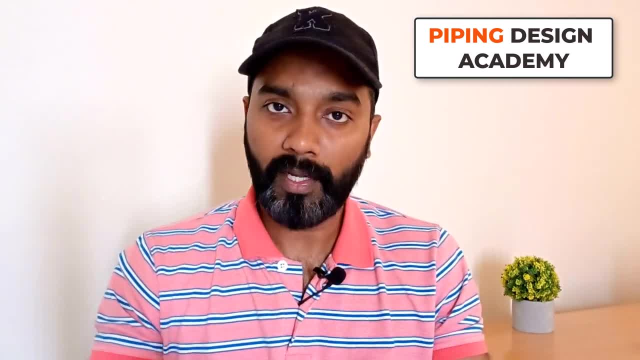 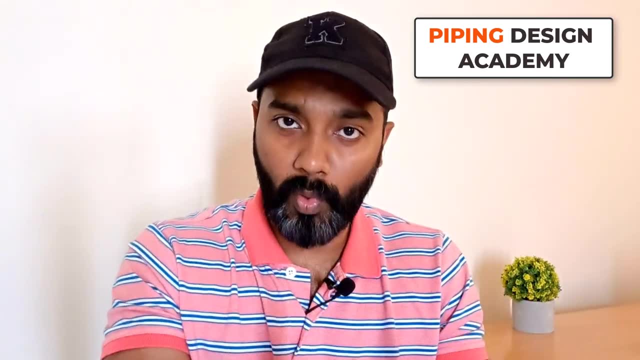 piping. you don't go and take up any course, don't take up any job. I mean don't choose your field. you have to understand this purpose. only if you understand the industries and your role and your job criterias and you will be able to feel that, whether it suits you or not, most of the people 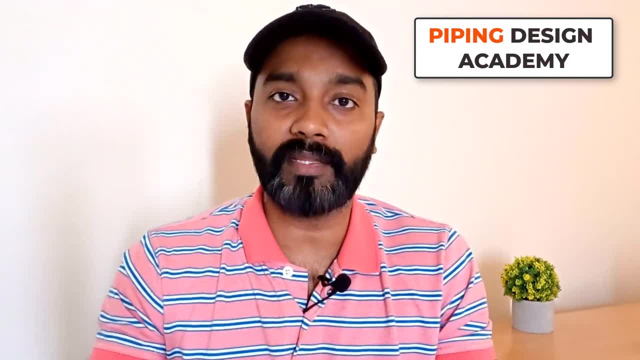 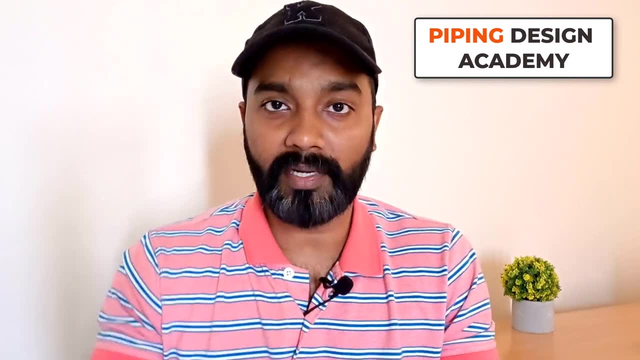 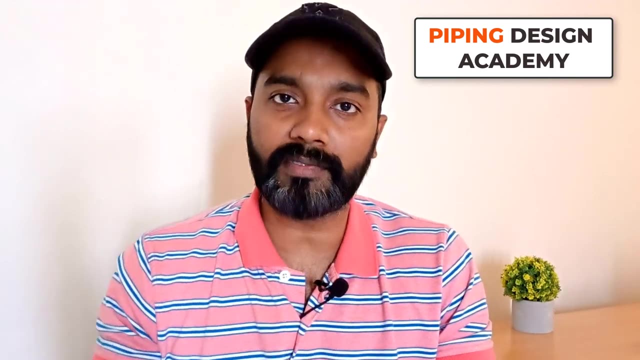 they choose piping design engineering just because? just because that they feel that it is easy to get into piping design engineering. that's not so. it may be easy to get into piping design engineering, but survival is the key factor for you, right? if you are not able to survive for longer period of time by losing an interest, then 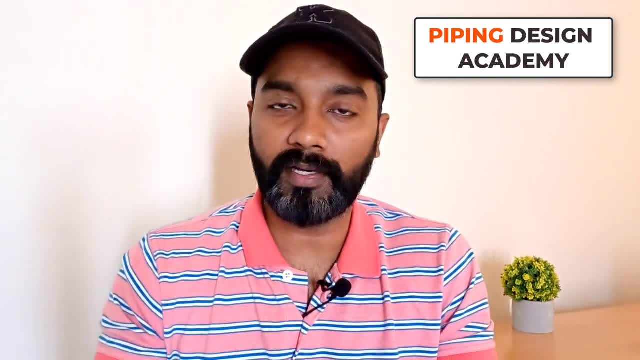 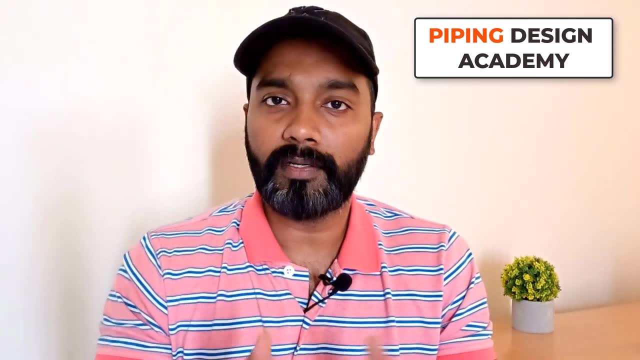 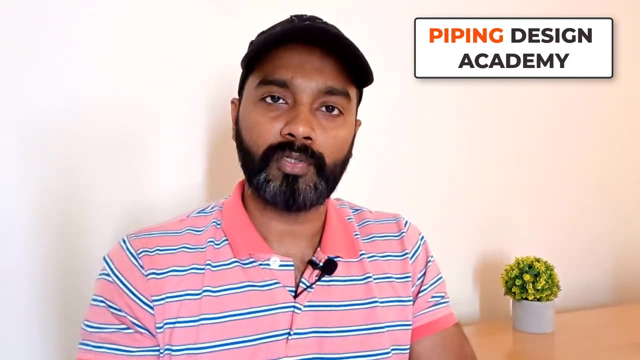 it's a waste of time, because your beginning years in your career is the golden time. don't waste that time. that I mean. I can only say that much actually be fruitful in using those times so that you can constructively grow from the day one actually. so that's very important. so now let's get into 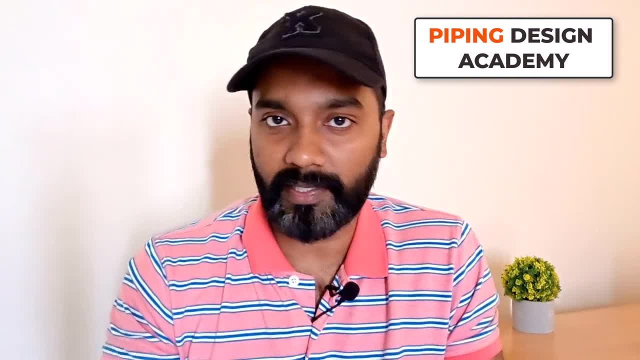 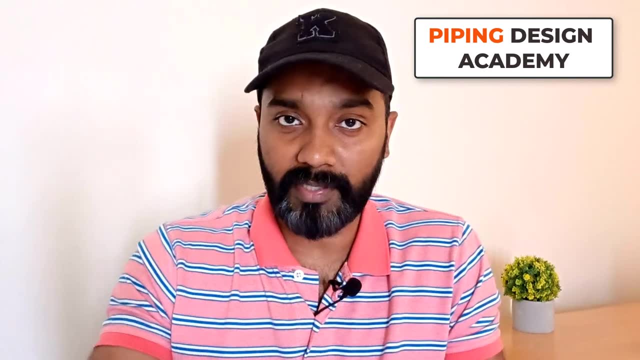 the basic requirements, the, what you have to prepare. basically, we have seen, you have to understand the purpose of the, your design, then you have to understand your responsibilities, then you have to understand the job criterias. now the fourth step is to understand the preparation, what you have to. 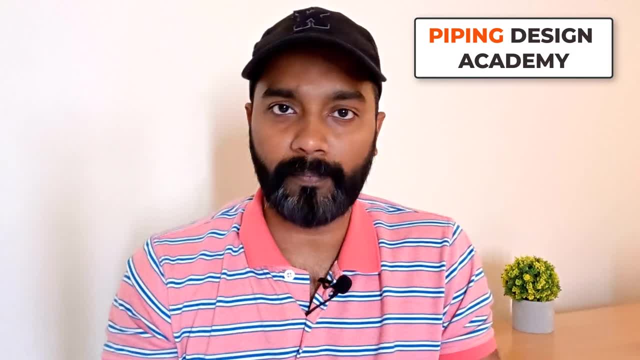 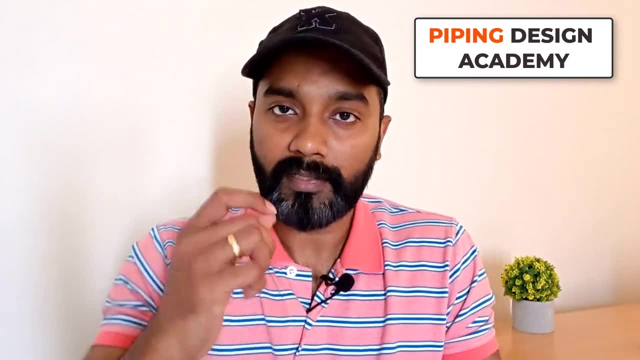 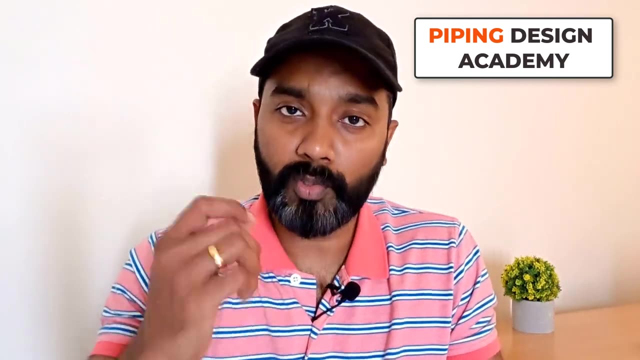 prepare, so that's the key factor that will help you to get a job. the first thing for any beginners to prepare yourself as a piping design engineer is that try to get some certification in the piping design course with this. let me just confirm you that do not spend more than 10- 15. 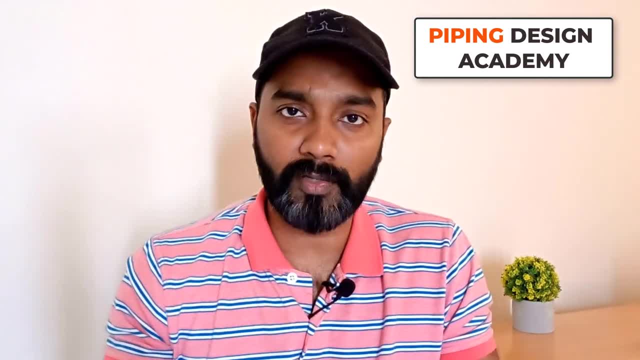 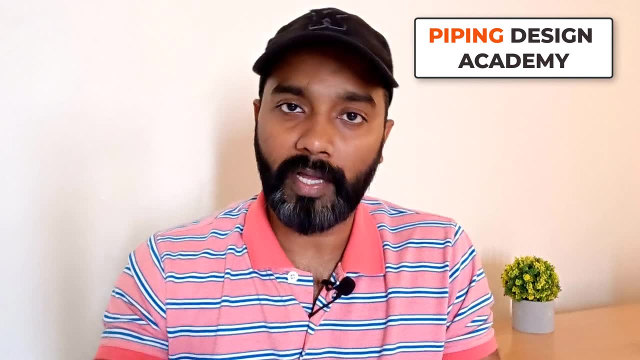 thousands of I mean it could be. it should not be more than 25 000 rupees because the certification is very important. certification will tell you that you have taken up a course and you know the basics of a piping design. that's the only requirement. I know there are people spending one and a half. 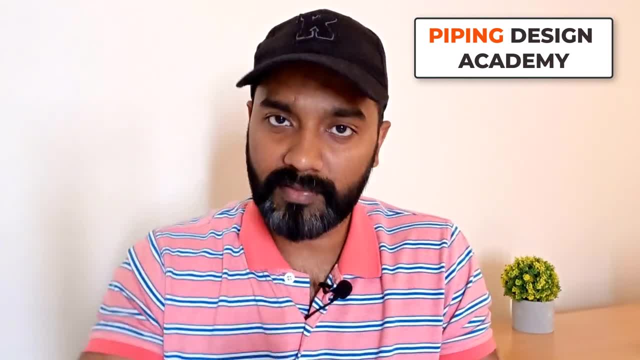 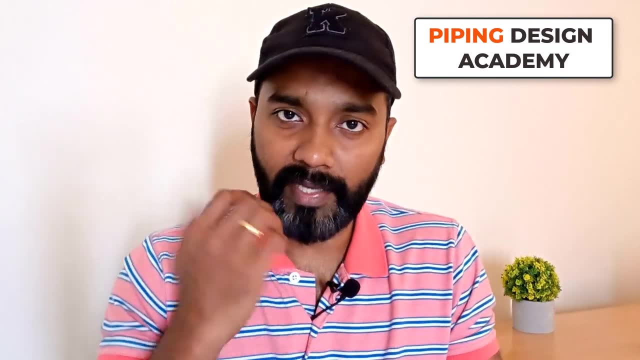 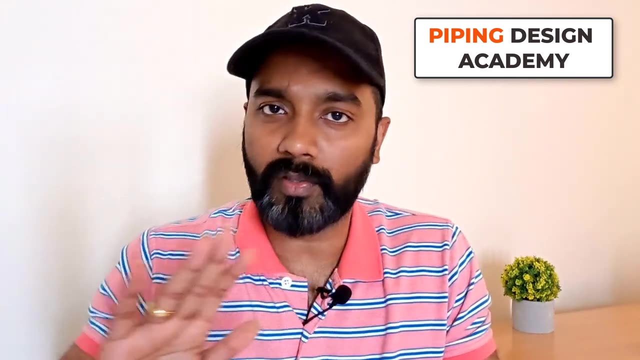 lakhs- two lakhs- to get this certification. but let me tell you, this certification will not have any value after two to three years once you get into this field. so this is exclusively for piping design engineers who are, as a beginner, for experience. these certifications are not going to do anything. 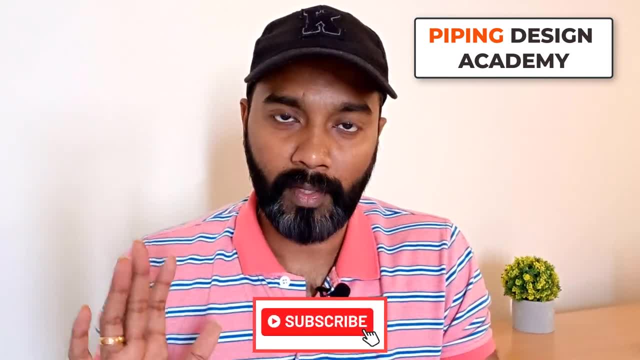 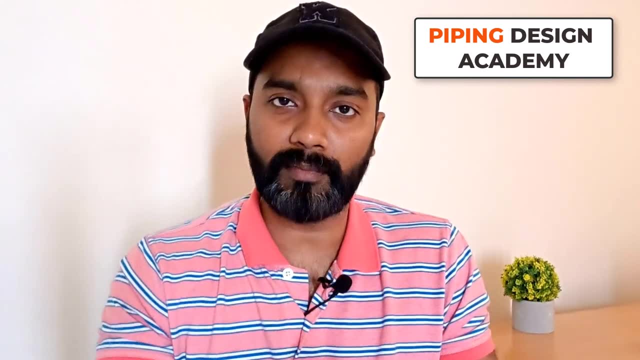 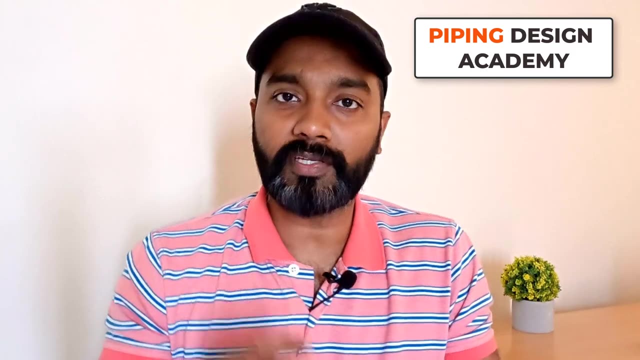 actually, whatever certificates that I have, it's no use. so do not spend the higher value, just spend not more than 25 000 and take a reasonable the theory classes so that you will be able to understand the workflow process of the piping design. so the certification is missed. so I would strongly prefer to take certification from any of your. 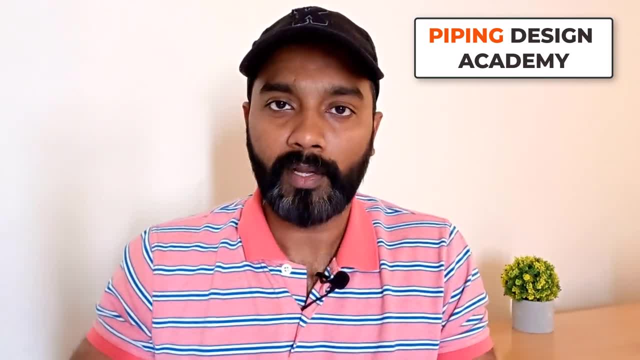 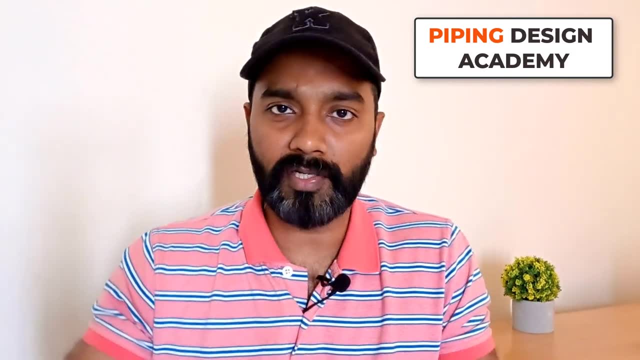 nearby institutes so that you can conveniently travel. don't take it from the other cities and spend a lot of time, money in accommodations and travelings. and all try to get a certification, because certification is just for a namesake, so that you can produce during an interview. 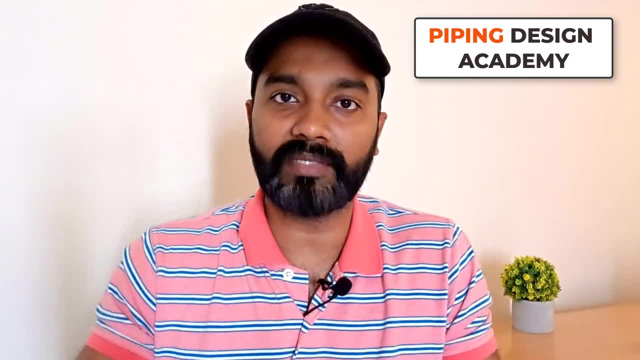 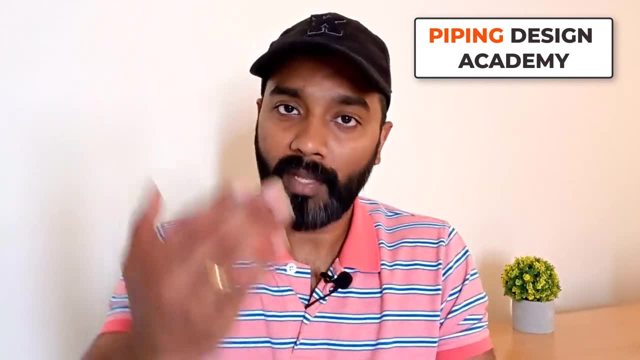 that will show. tell the interviewer that you have done some basic work in piping. so that's the importance of the certification. this is first one, and the second requirement is that self-study you have to do. so what is the self-study you have to do? first thing, try to learn. 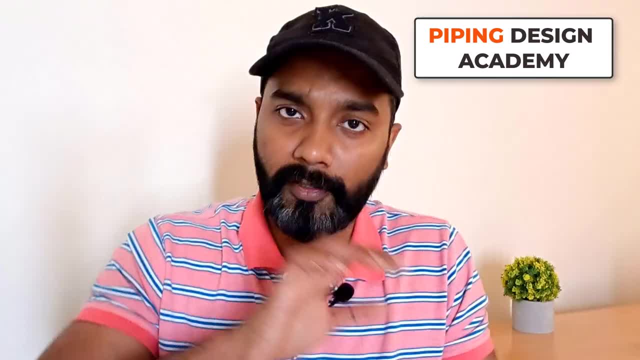 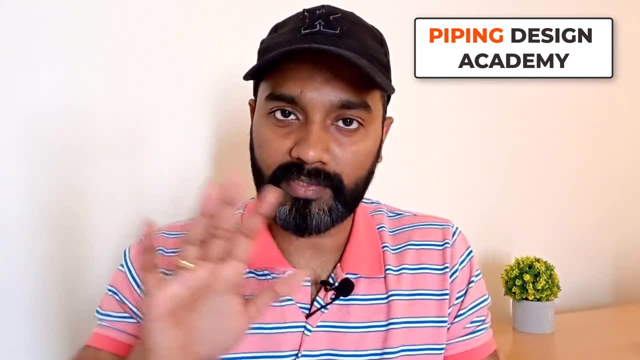 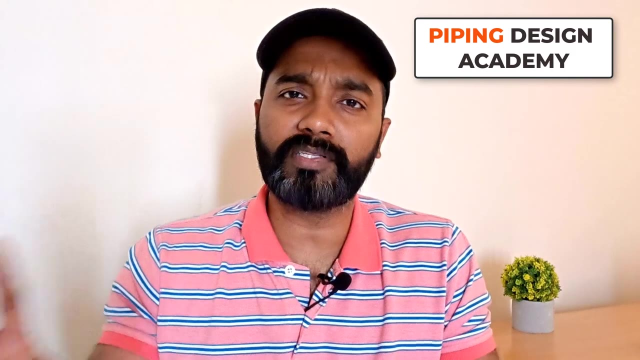 each and everything about pipes and fitting details. there are different types of pipes are available. different types of fittings are available. you have to thoroughly, you have to buy hard all these things there. what is the standard? what is the dimensional standard? what are the different types of? what is the purpose where we are using all these informations are available in the internet. 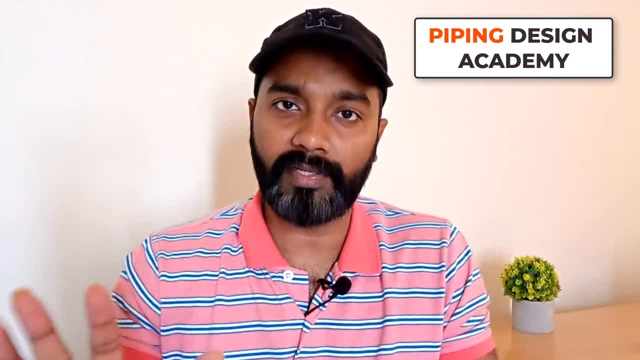 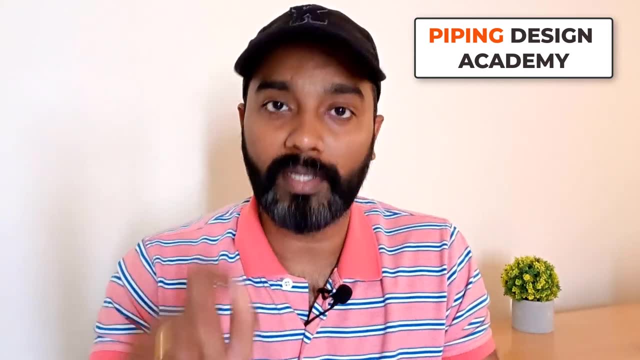 you don't have to spend any money for that. it's completely free of materials which are available. even in my channel i have explained about pipes and fittings and in standards and everything actually. but you have to know this information- pipes and fittings- clearly. you have to clearly. 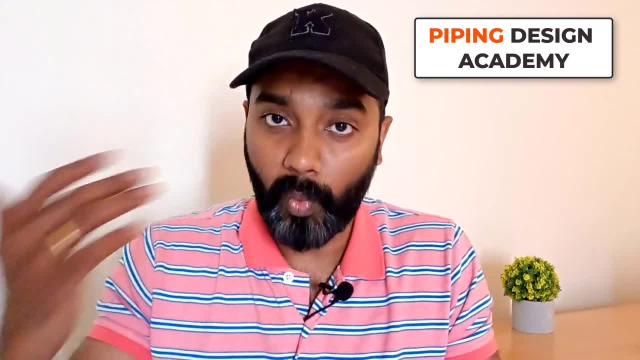 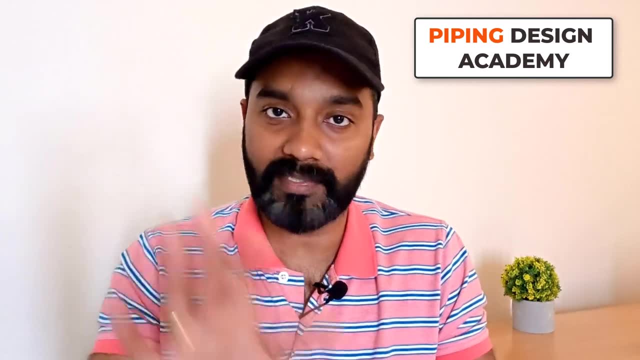 i have to aware about each of these categories with what is the standards of fittings? what are the dimensional standards? what are the difference? these things you have to have. so just the basics you have to aware. as a beginner, nobody will question you about the depth of standards or 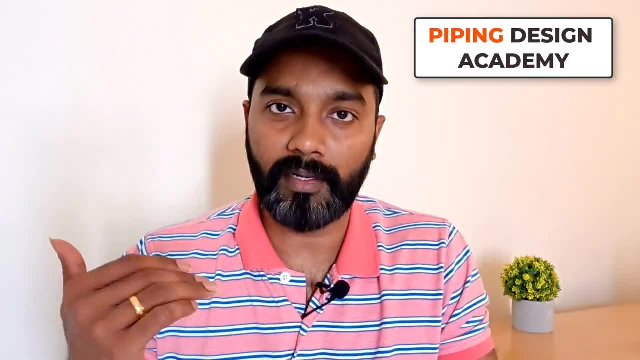 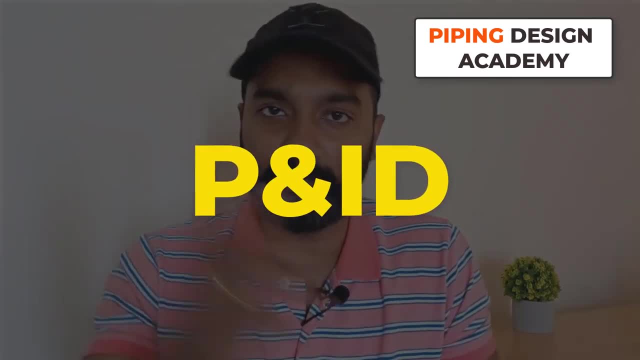 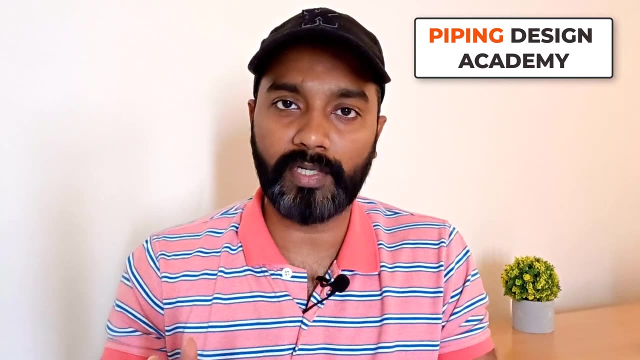 depth of in your design requirements as a beginner, only you. we are expecting you to have this knowledge right now. the third important thing is that pnid reading is: must you have to learn how to read the pnid as a beginner? this thing, you, it is very must for you actually, again, once again, there are lots. 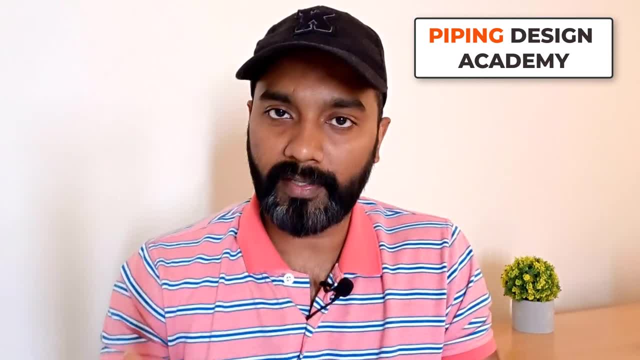 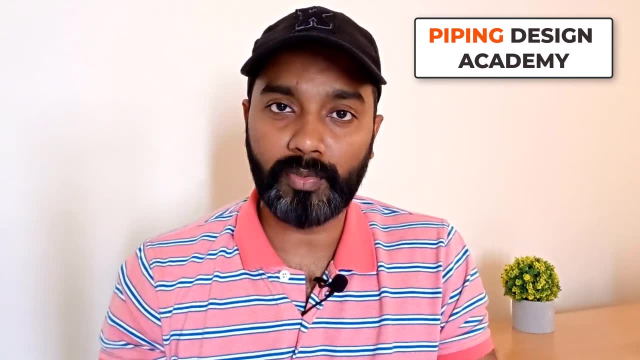 of materials available. even in my channel it is available. i can even give you a link about that particular videos in the description box. but the vital, key factor message that i wanted to share is that don't skip the pnid reading. pnid reading is the must for pnid reading and pnid reading is the 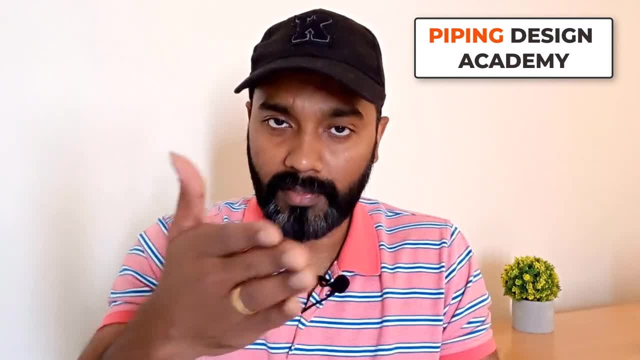 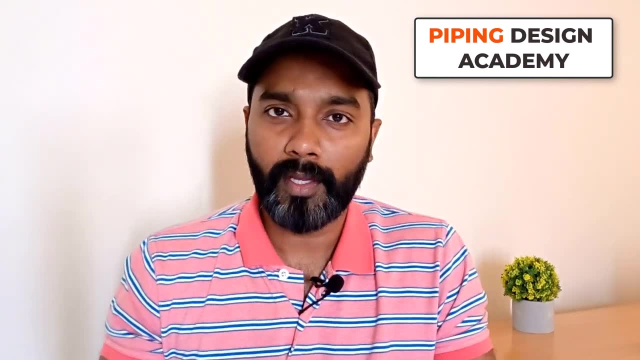 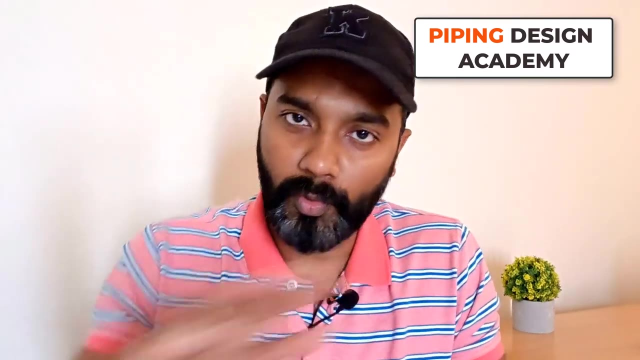 must for beginners in piping. so you have taken a certification, then you have read about pipes and fittings, and then you have read about pnid. now the fourth thing is that you have to understand pipe routing and pipe support, which is the key role for any piping design engineers. if you do, 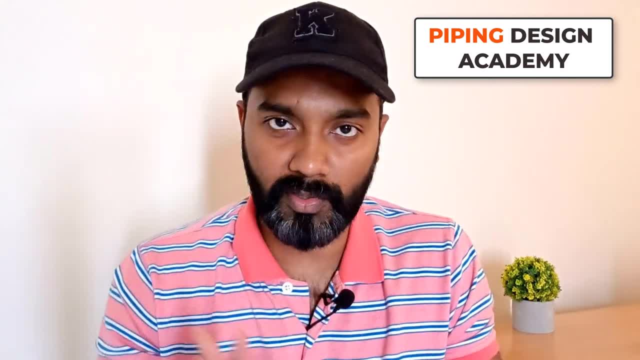 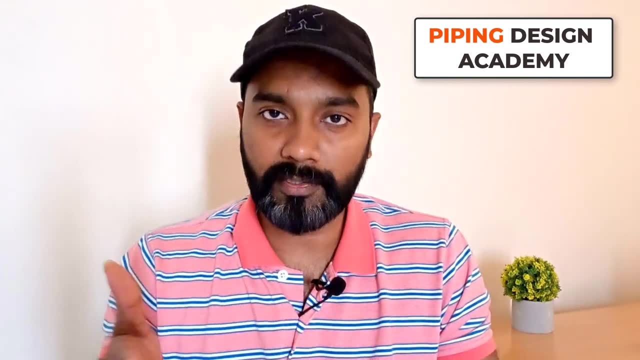 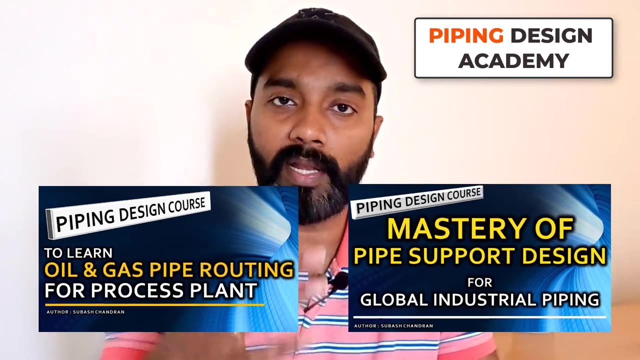 not know pipe routing and pipe supporting placement, then you cannot consider yourself as a piping design engineer. even i have two wonderful courses. you can check those details of the courses in my website, which is a pnidcom, the link i'll give you in the description of this video. these courses will help. 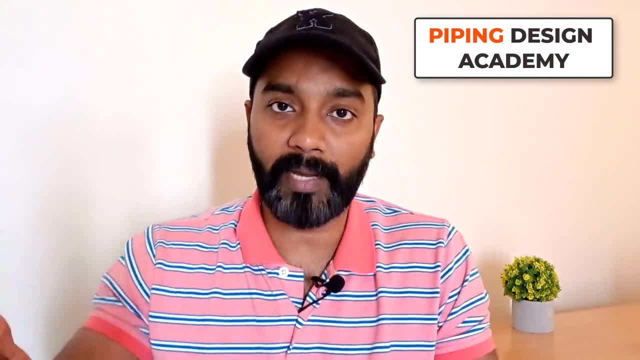 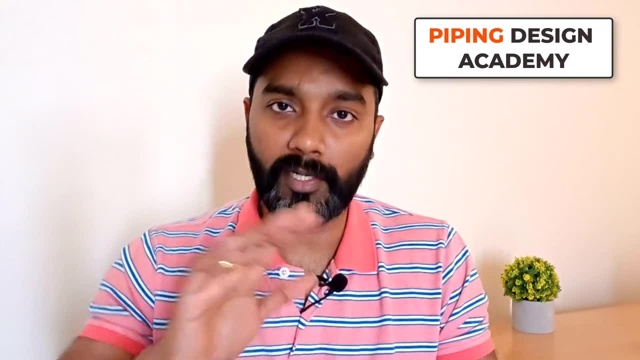 you to develop the skills that are required for pipe routing and pipe support placements, which are actually needed for a real-time job. this is not just a theory. in this course, i have explained the logics, concepts and how to take decisions. what are the engineering specifications? what is the minimum requirement that you have to meet for these? 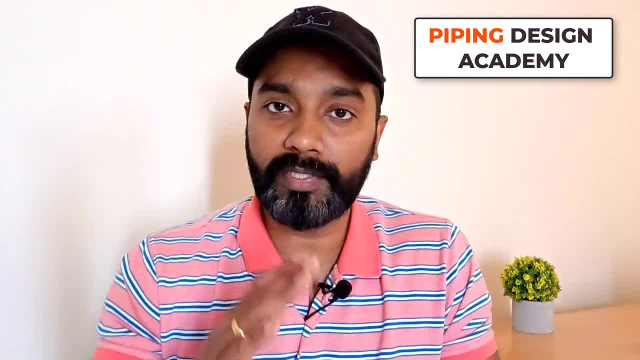 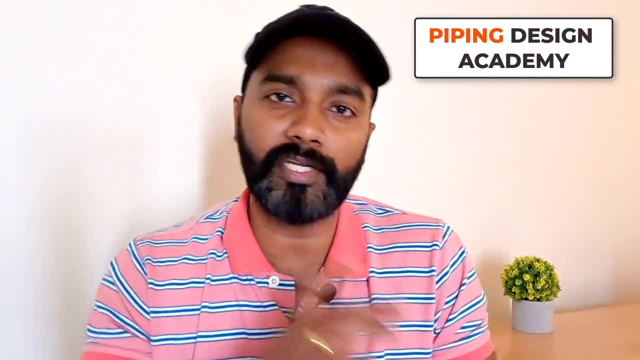 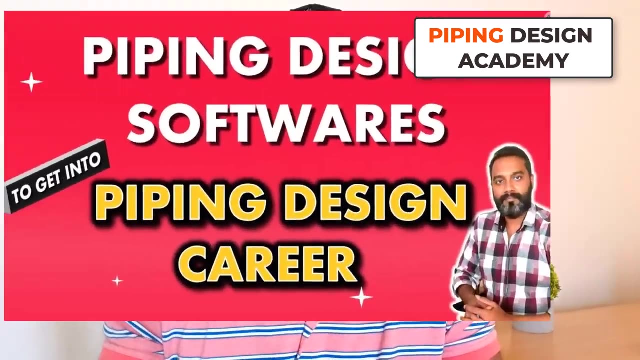 routings and supports. so these courses will help you to develop these two skills- pipe routing and- and the next requirement that you have to have is that 2d and 3d tools. there are 2d tools and there are 3d tools. i have also made a video of these 2d and 3d tools. i'll 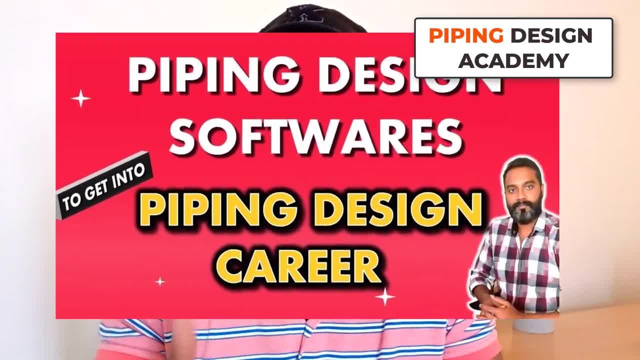 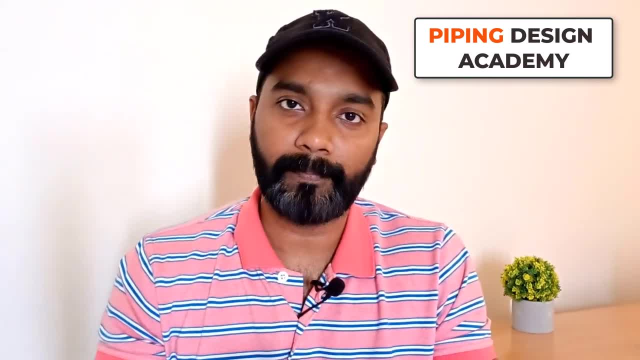 share you the link of this, but 2d and 3d tool requirements is a must for beginners. so these are the five set of preparation that you have to do as a preparation, basically because these are technical areas, but you have to be really strong in these five areas that i've. 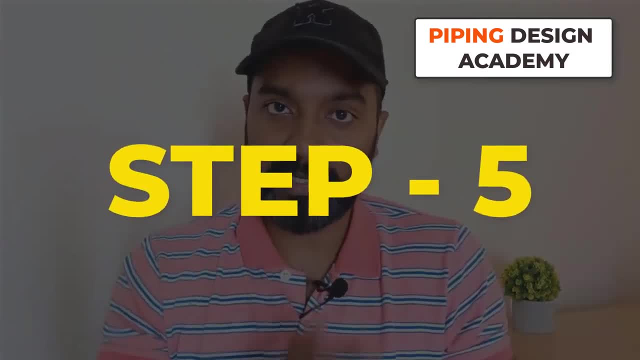 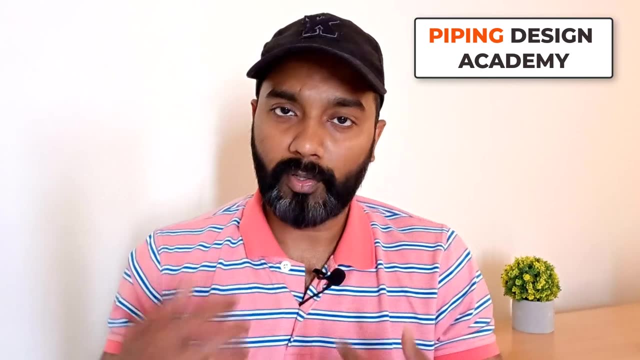 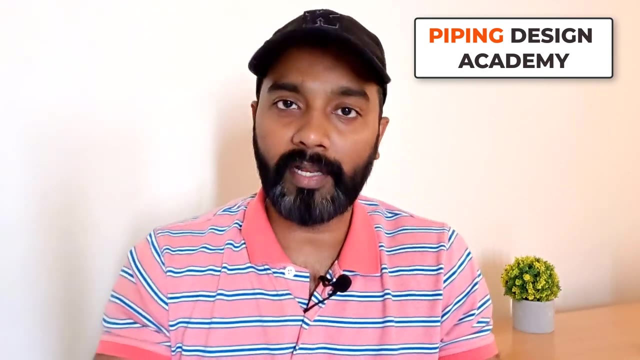 told you just now, actually, and the last stage and the last stage is what you have to deliver as a piping design engineer. that you have to understand, right, because you are a piping design engineer and you want to understand what you have to deliver. you know the industries and you have prepared and everything but. 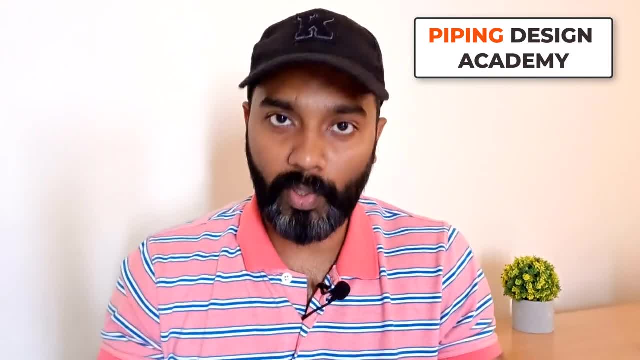 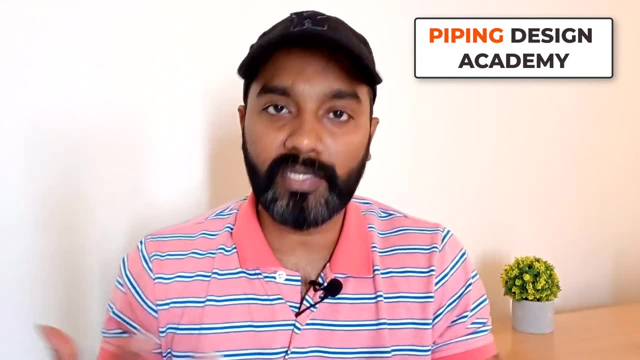 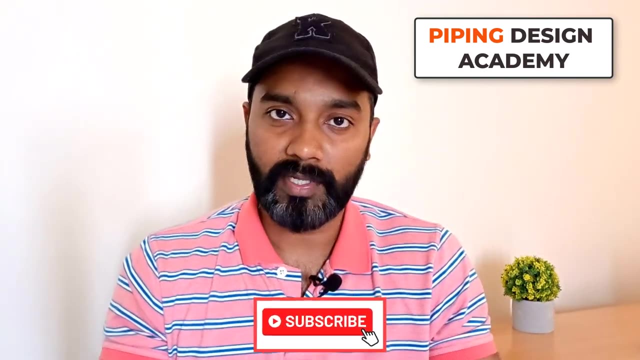 what you have to deliver, that you have to understand. you have to deliver that drawings such as plot plan, piping, layout, isometrics, empty who's pipe supports. these are the basic requirements, deliverables that you have to submit: engineering packages and bulk MTUs and the iso-wise MTUs and fabrication isometrics. 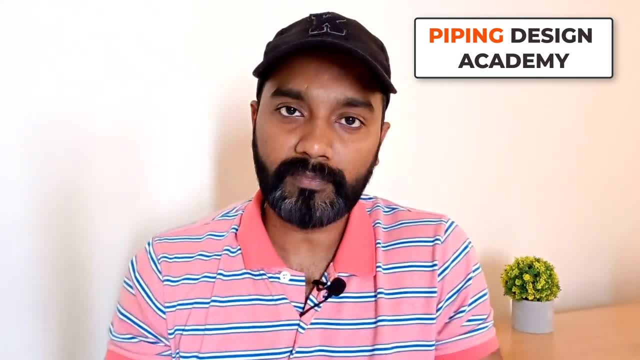 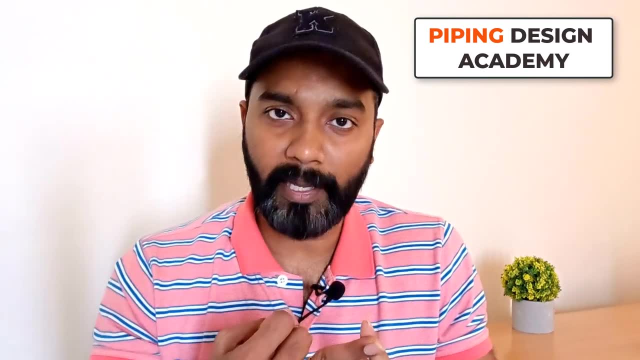 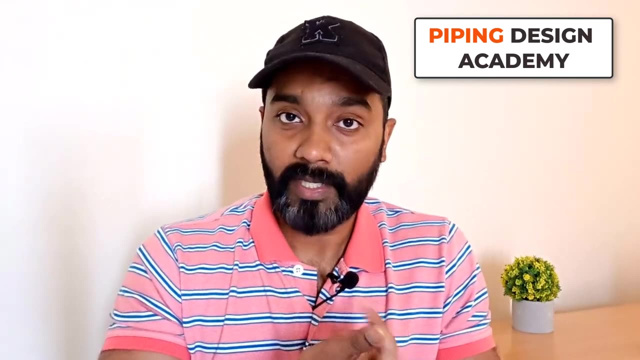 there are n number of derivatives are there that you have to understand. So let me tell you the few important things that you have to understand. One is plot plan, another one is piping layout and piping isometrics, then pipe support drawings, then bill of materials. Just focus on these five important areas First, as a beginner, 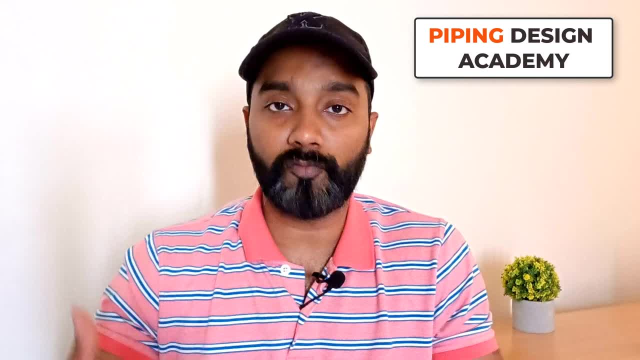 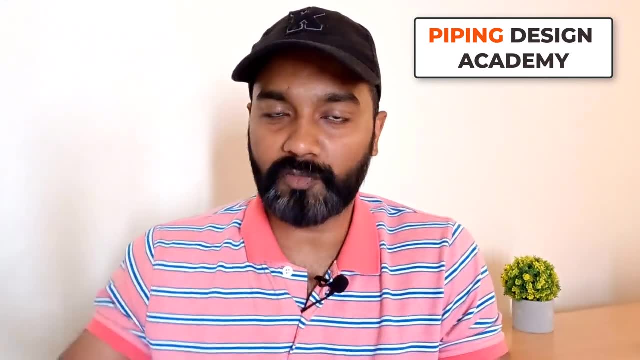 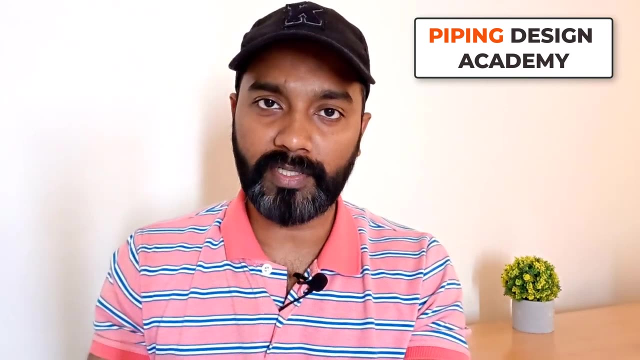 that is enough for a beginners to get prepared for any job Because, as a beginner, industry knows that they cannot expect you like they can expect from the experienced person. So these are the key, important things that you have to learn. If you learn these key, important things, then 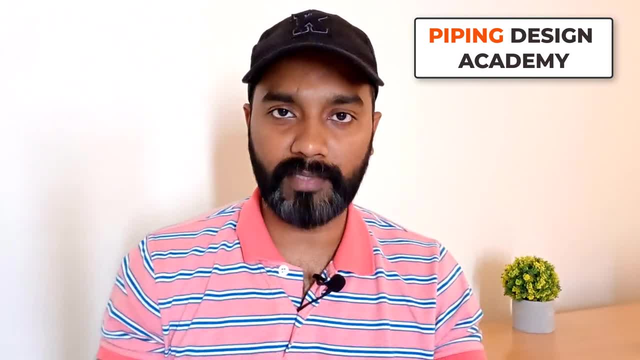 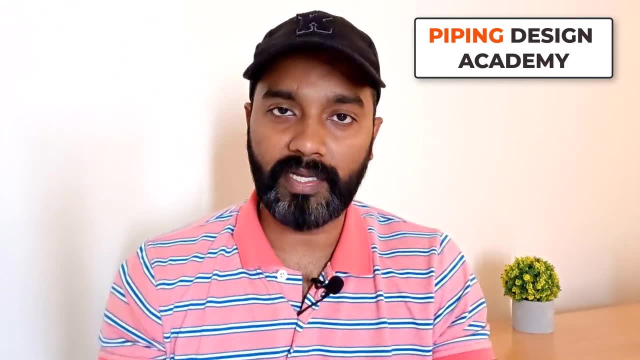 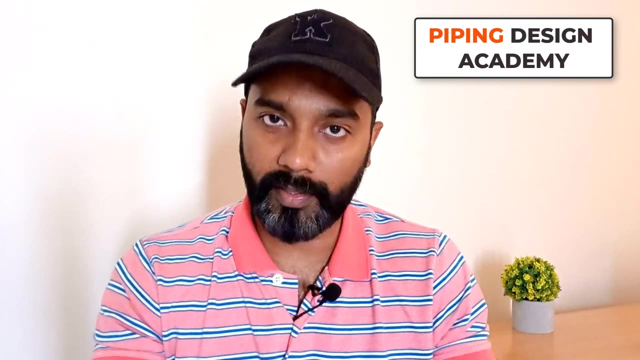 you will be qualified to get into a job. Don't waste in some areas which is completely not useful to you. One of the advice that I would share with you is that and you can start reading books. I can share those must read books that I have already made a video on that, actually. 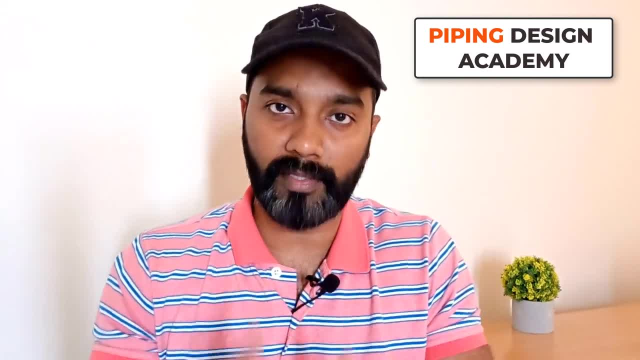 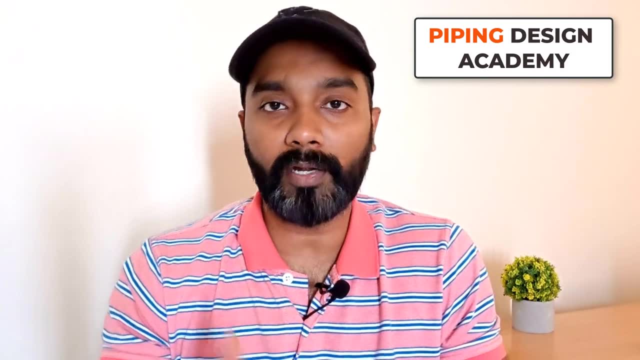 So that will give you an idea about what books that you have to read in order to gain the knowledge Reading inputs that you have to keep it as a side, actually, because that should be a part of your daily life. So you have to spend at least half an hour to one hour If you can.